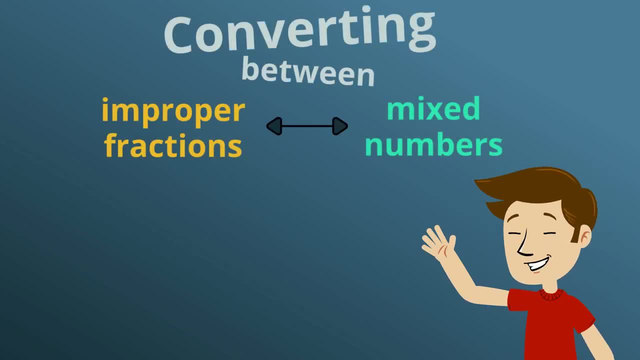 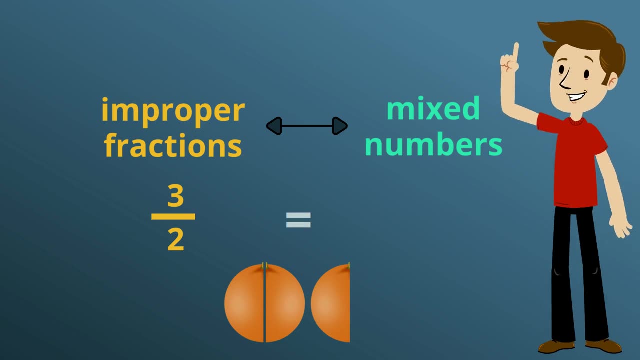 Converting between improper fractions and mixed numbers. This video assumes an understanding of the connection between improper fractions and mixed numbers. If you'd like to review this, check out our video on this topic using the link in the description. Before we start looking at how to convert between improper 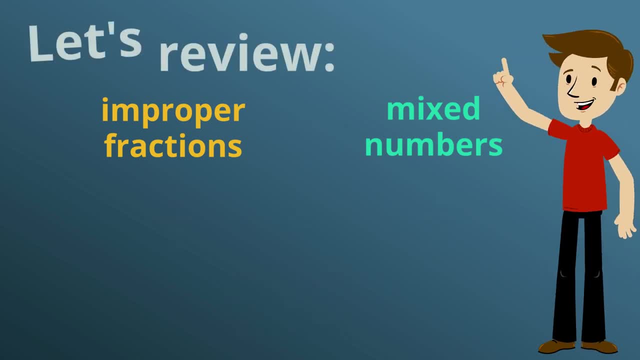 fractions and mixed numbers. let's quickly review what each is. An improper fraction is a fraction with a numerator larger than its denominator. For example, three halves. Improper fractions are greater than one. A mixed number is a mix of a whole number and a fraction. 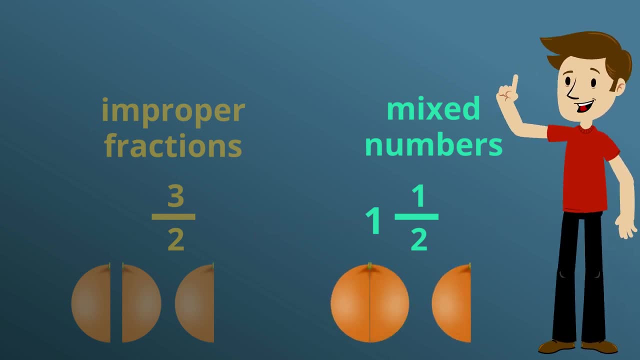 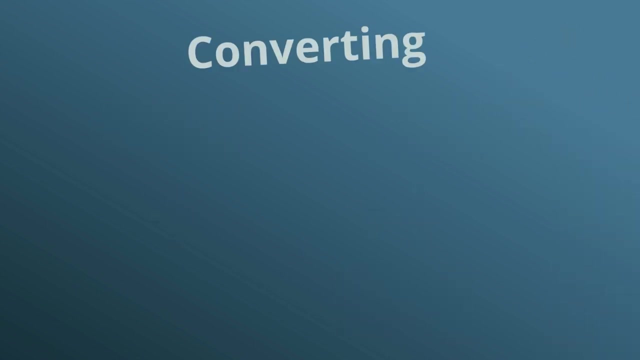 For example, one and a half Mixed numbers are also greater than one. You can see here that three halves and one and a half are equivalent. Let's look at how we can convert between the two. We'll start by converting a mixed number, two and a quarter, into an improper fraction. 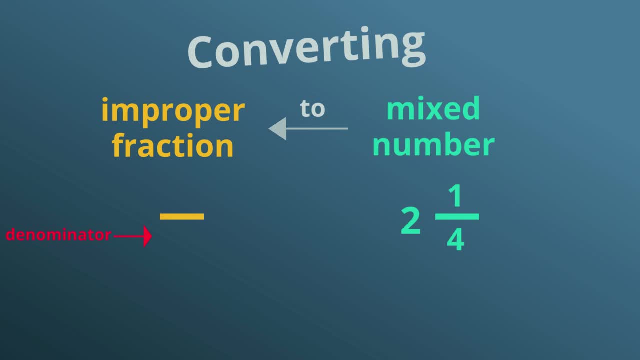 First we write down the denominator of the improper fraction. Because our mixed number is in quarters, our improper fraction will also be expressed in quarters. Then we multiply the whole part of the mixed number by the denominator. In this example, that's two multiplied by four, which is eight. 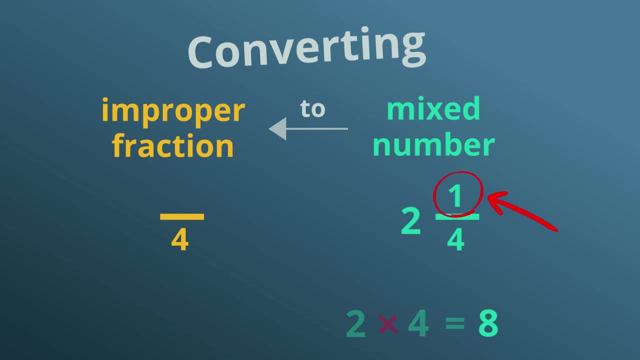 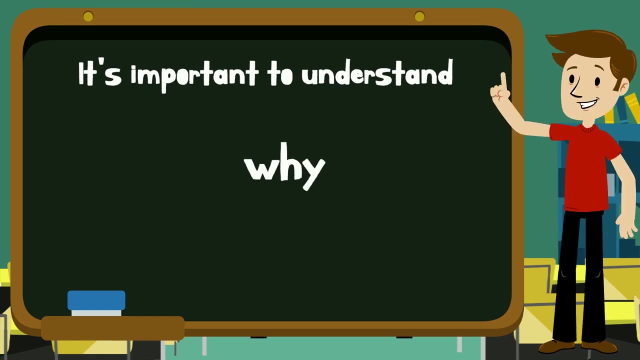 Then we add the numerator, which is one, to this number. Eight plus one is nine. This is the numerator of our improper fraction Two and a quarter, as an improper fraction is nine quarters. It's important to understand why we follow these steps, so let's go back and take a closer look. 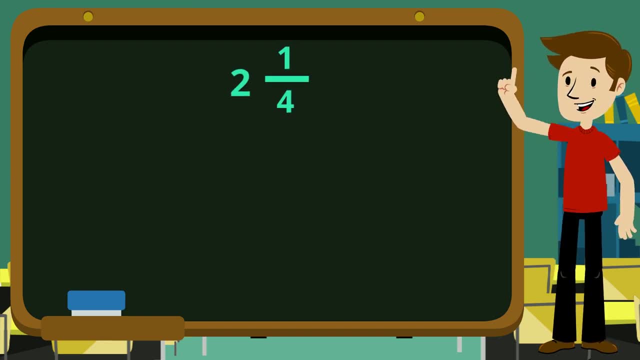 Here is the mixed number we started with. Why did we multiply the whole part of the mixed number by the denominator? Because if we're working with quarters and we've got one whole, how many quarters do we have altogether? That's right. four: 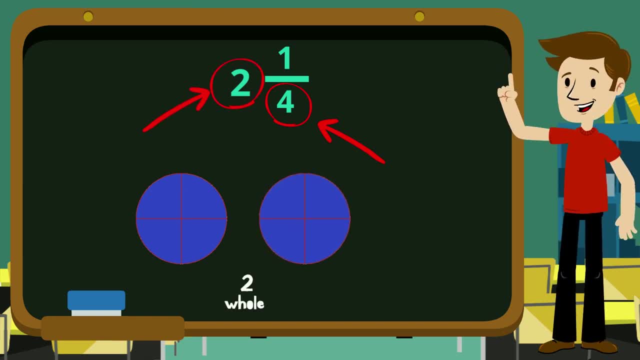 So if we've got two whole, how many quarters would we have? Eight, because two lots of four is eight. Now this means the number of quarters is an odd number. So if we multiply this number by twice, that is one quarter. 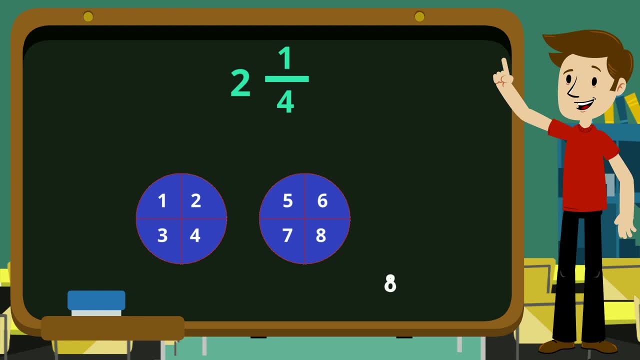 That will add up to eight. So in the next step we added the numerator to this number. Why? Well, so far we have eight quarters. Now, eight quarters is simply two whole, but the mixed number shows us that, as well as the two whole, 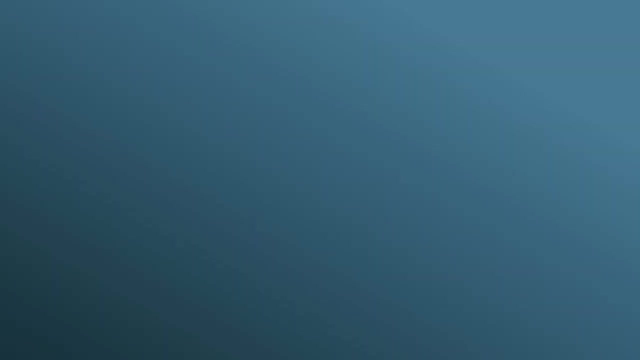 there is another quarter, So we add the one quarter to our eight quarters. back the other way, converting an improper fraction to a mixed number. To help you understand the process, we'll use the improper fraction: 9 quarters. First we must work out how many times the denominator fits into the numerator. 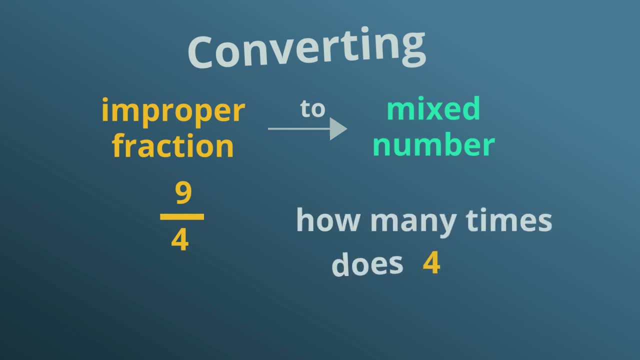 That is, how many times does 4 fit into 9?? We can see that 4 fits into 9 once. twice. it fits in two times. This becomes the whole of our mixed number. Since the improper fraction is in quarters, our mixed number will also be in quarters. 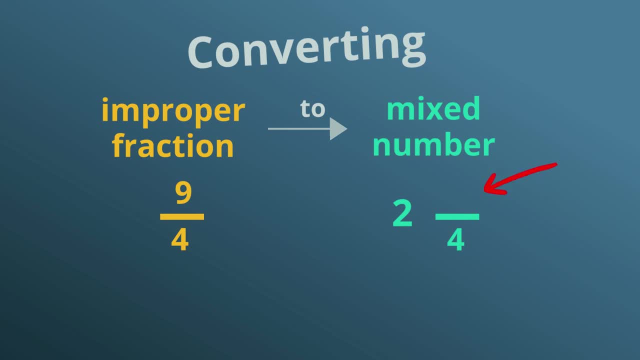 All that's left is working out the numerator of our mixed number. When we worked out how many 4s fit into 9, it didn't fit evenly. There was 1 left over. This 1 becomes our numerator, 9 quarters as a mixed number. 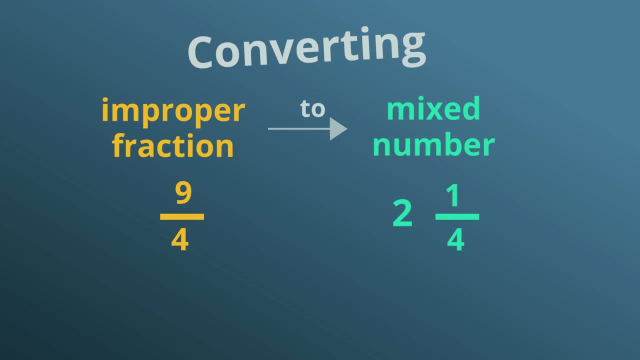 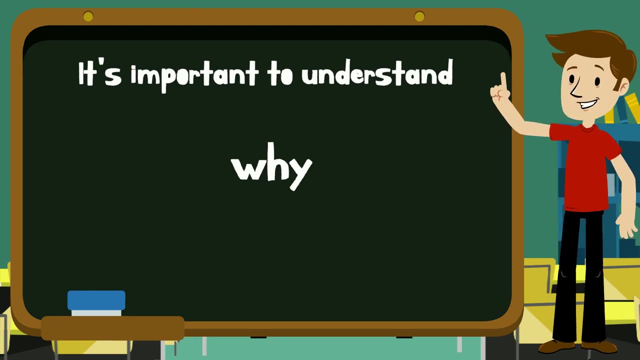 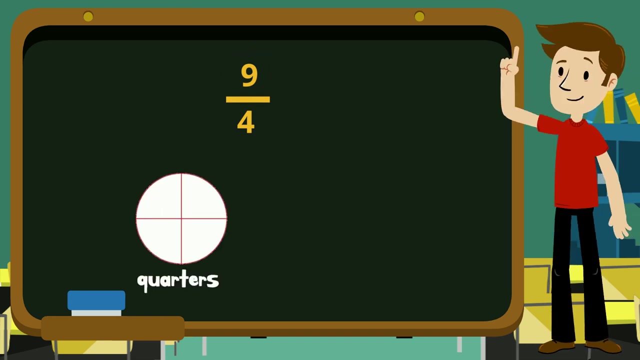 is 2 and a quarter. Again, it's important to understand why. so let's go back and take a closer look. Here is the improper fraction we started with. Why do we work out how many times the denominator goes into the numerator? Well, since we're working with quarters, 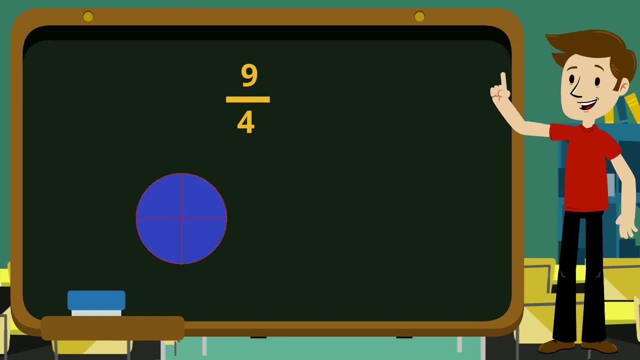 we know that every time we have 4 of them we have 1 whole. So by working out that there are 2- lots of 4 in 9, we know that our number must have 2 whole. Then we get our numerator. 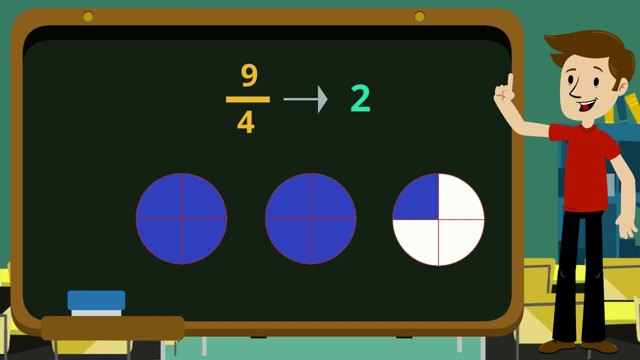 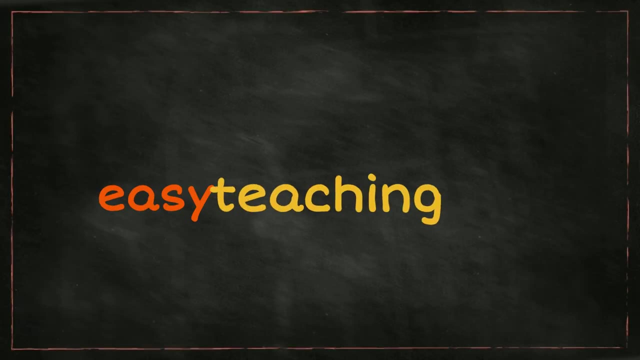 from the number left over, because, while there weren't enough quarters left to make a numerator, a new whole, it's important that we don't forget that this single quarter is also a part of our number. Thanks for watching EasyTeachingnet.